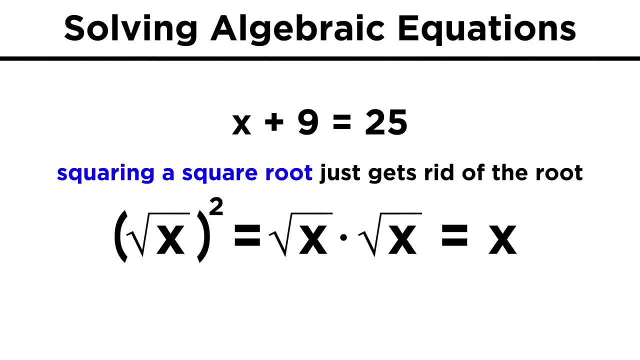 That gives us x plus nine equals twenty-five. To really prove that squaring a square root gets rid of the root, let's remember that taking the square root is the same as raising to the one-half power. so we can rewrite this equation like this: 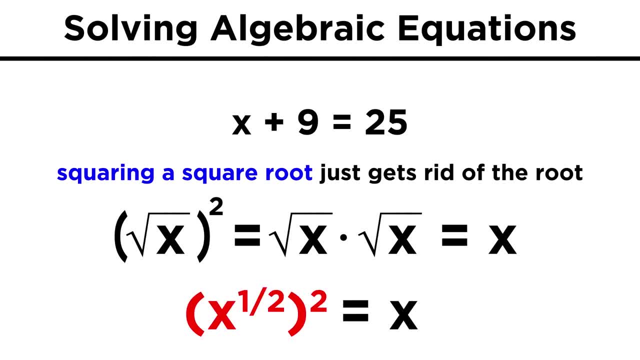 On the left we have this term to the one-half power, to the second power. We can recall from our rules of manipulating exponents that x to the a to the b equals x to the a times b, And here a times b or one-half times two equals one. 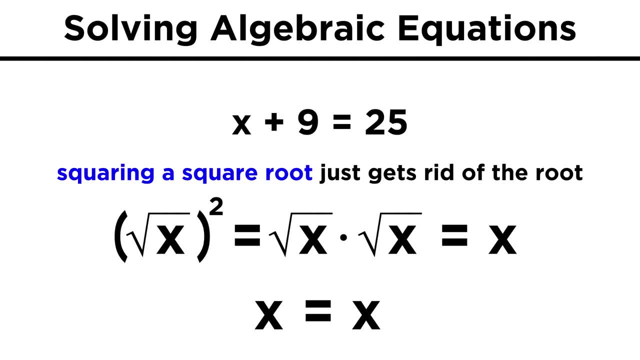 So the one-half and the two essentially negate one another, to just leave the term by itself. Now things look much simpler: X plus nine equals twenty-five. so we subtract nine from both sides and we get x equals sixteen. How about something a little trickier? 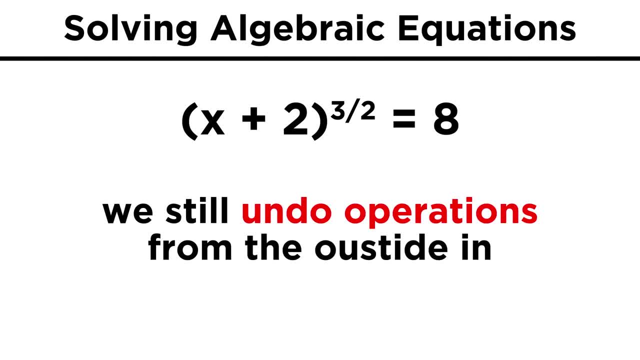 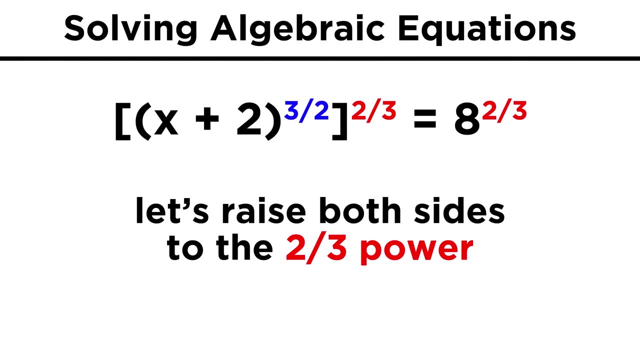 We still just go from the outside in undoing every operation that acts on the variable. we are solving for one at a time. First, we have to get rid of the exponent. How do we get rid of the three halves? The fastest way to do it would be to raise both sides to the two-thirds power. 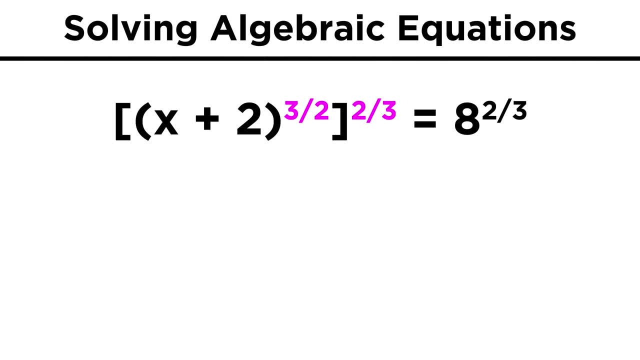 If we raise this term, that is, to the three halves, to the two-thirds power, we are raising it to the three halves times two-thirds power And if we do this, it's going to be the same thing: We're going to get rid of the exponent. 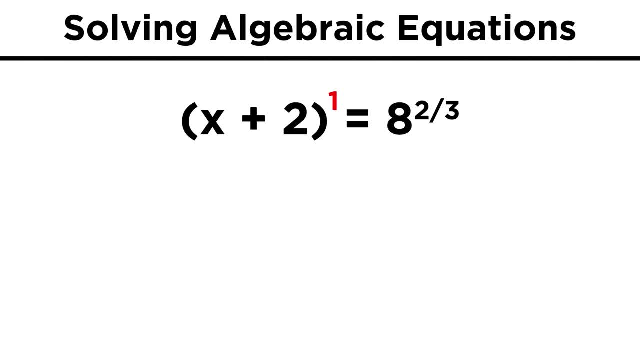 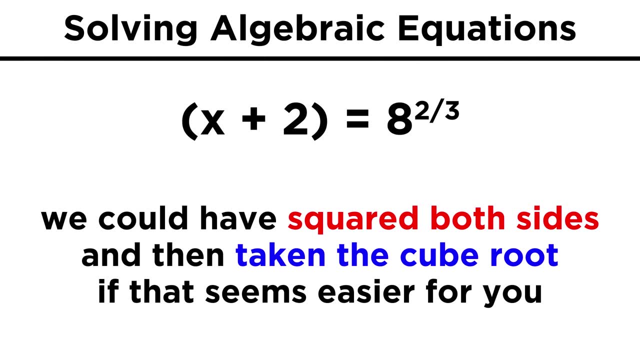 Everything cancels and we just get one as the exponent. Another way to do it would be to square both sides and then take the cube root. but why do two steps when you can do one? Now, on the right, we have eight to the two-thirds. 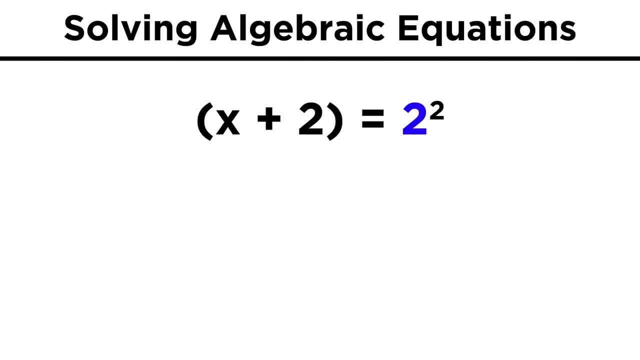 This we can just evaluate by taking the cube root, which is two, and then squaring to get four. Now we are left with x plus two equals four. so we just subtract two from both sides to get x equals two. When we have something like x squared plus five equals forty-one. this is also quite. 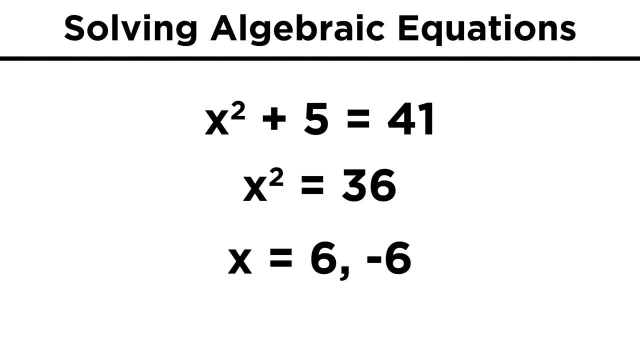 easy. We just subtract five and then take the square root. But remember, when we take the square root of something we get two answers, in this case positive six and negative six. so we have to keep in mind that these types of equations